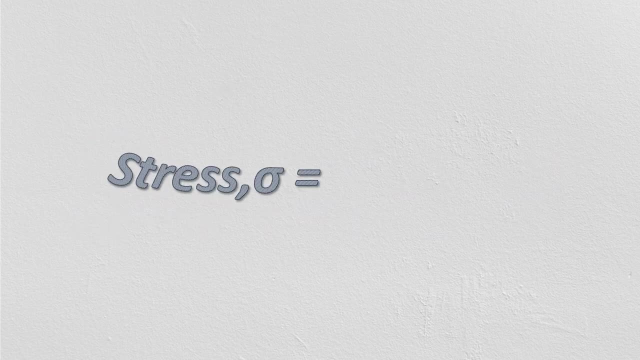 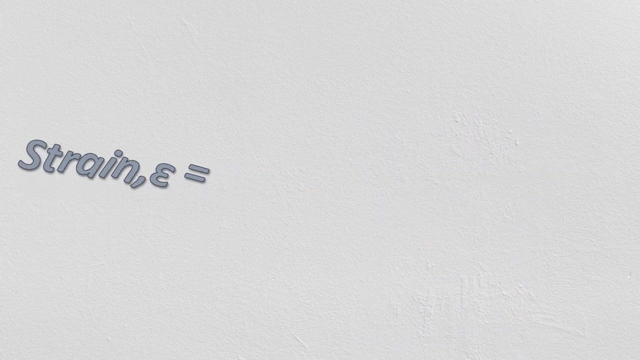 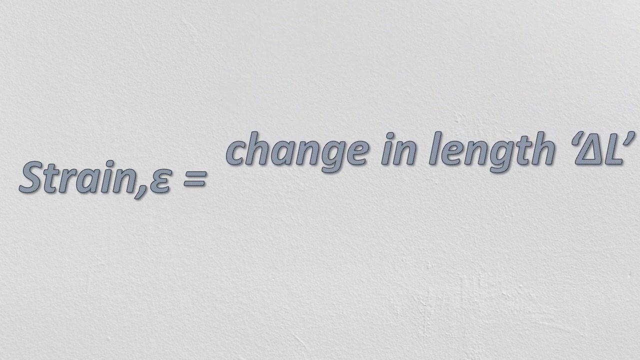 stress and strain In tensile test. stress is calculated as load applied to a material divided by the cross-sectional area of the material. The strain is the deformation or displacement of material due to applied load and can be calculated as change in length divided by original length. In Stress Strain Curve, the stress is shown. 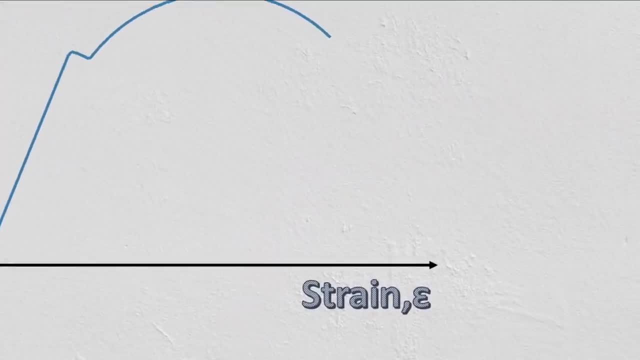 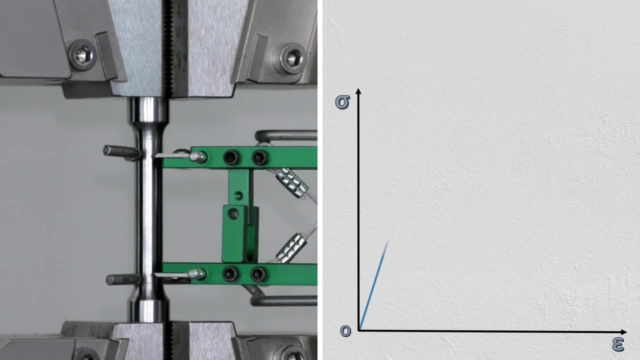 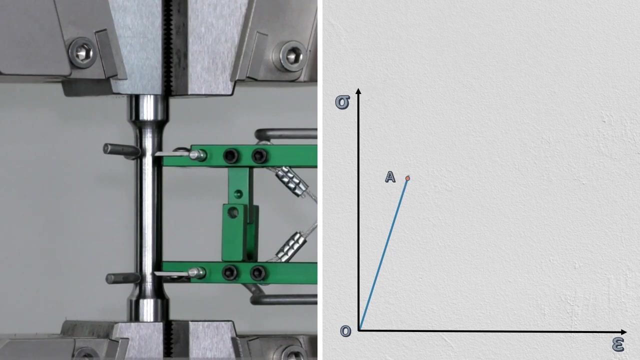 along the Y-axis and strain is shown along the X-axis. As we load the testing object in Tensile Test test, it begins to deform and stress continuous to raise linearly up to a point A on this graph. At this point A, if we remove the applied load on the testing object, it will restore. 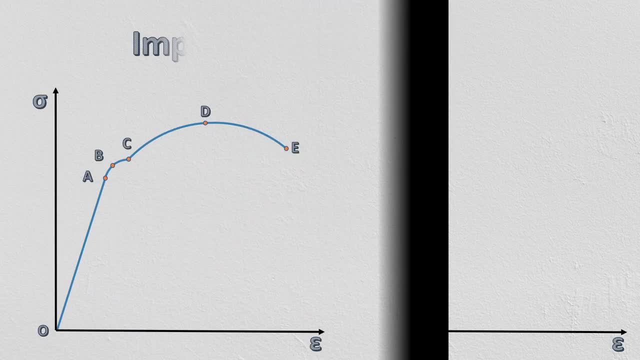 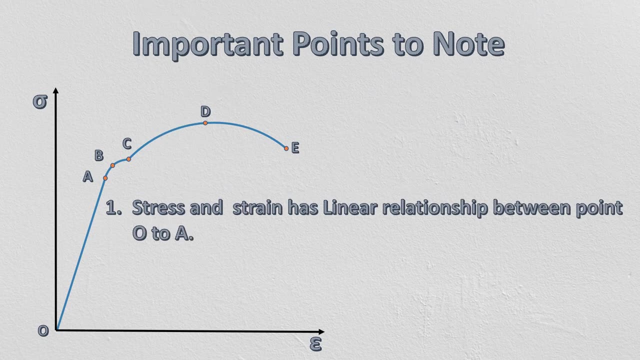 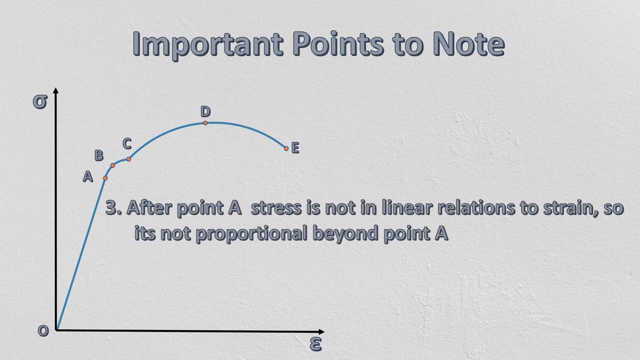 to original shape without any deformation. As you can see in this graph, from point O to A the stress and strain has a linear relationship And stress is directly proportional to the strain within this region. At point A, the proportionality between stress and strain no longer exists, hence the stress. 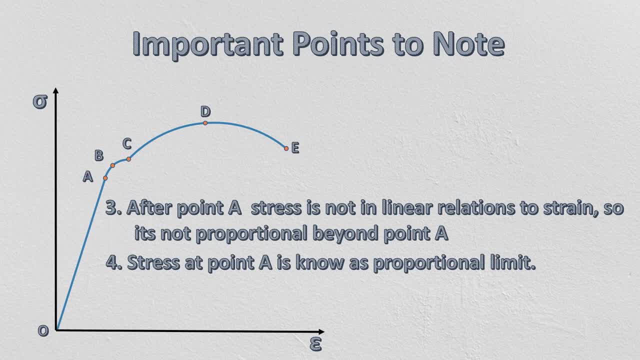 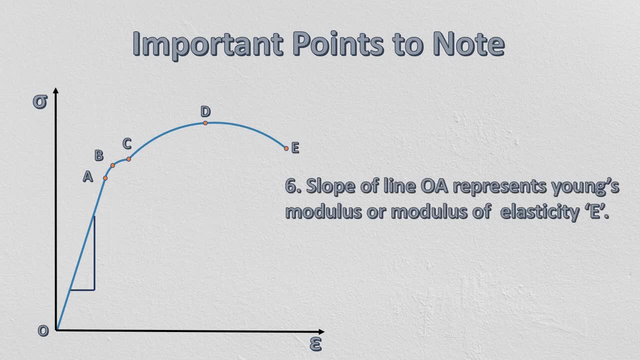 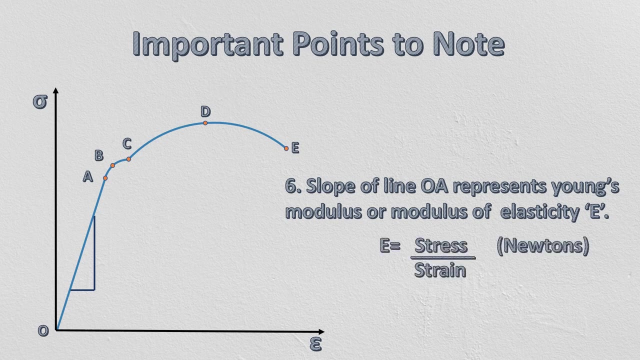 at point A is called the proportional limit. The Hooke's law is valid up to this point only. The slop of this line O A represents the Young's modulus, also known as modulus of elasticity, And it can be calculated as stress divided by strain within proportional limits. 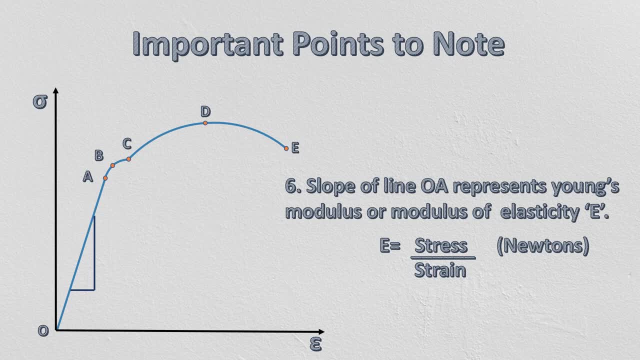 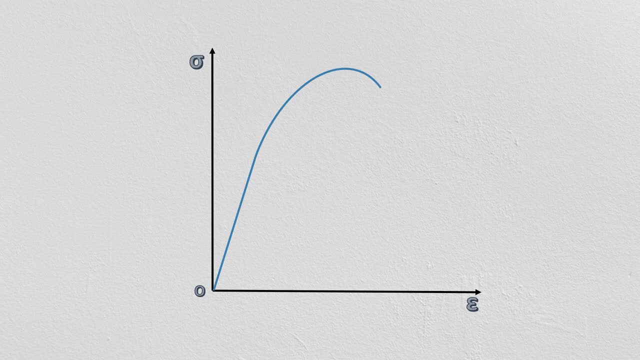 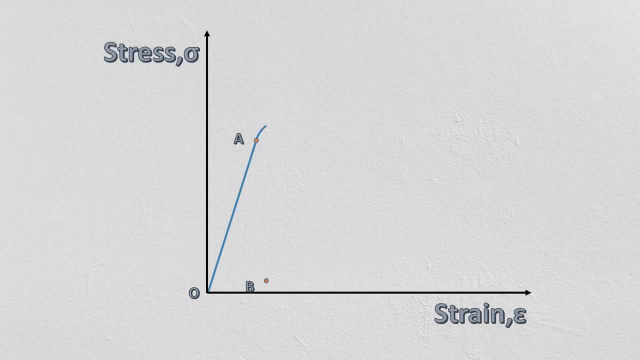 Higher slope means stiffer and stronger material. for example, High carbon Steel and its curve will look like this, Whereas for flexible material like elastomers, curve will look like this. Remember, these curves are not to scale With increase in stress beyond the proportional limit, strain being to increase more rapidly. 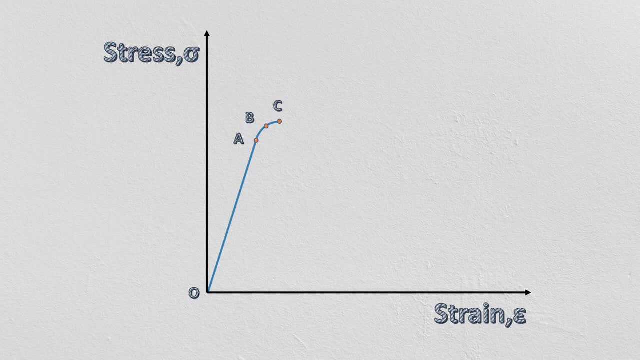 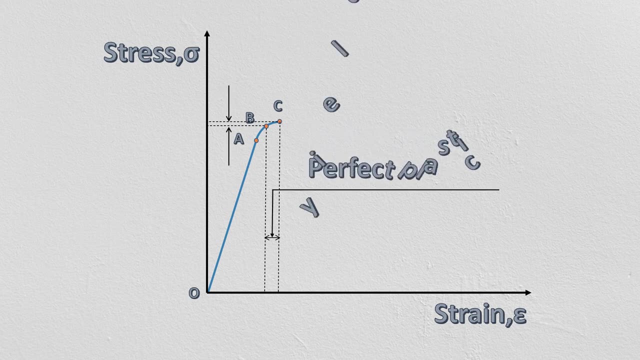 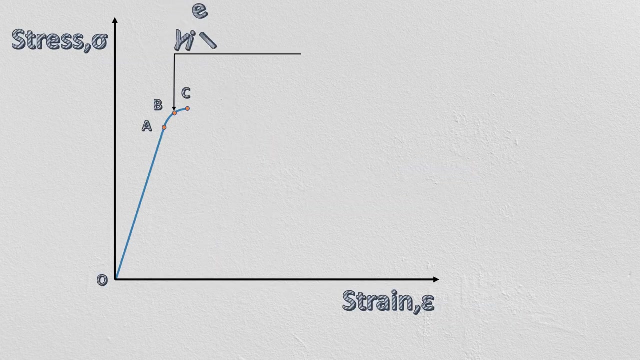 for each increment in stress From point B to C, there is considerable increase in strain without much increase in stress. This is because of plastic deformation in the metal, And this phenomenon Is known as yielding. The point B, where this yielding begins, is known as the yield point. 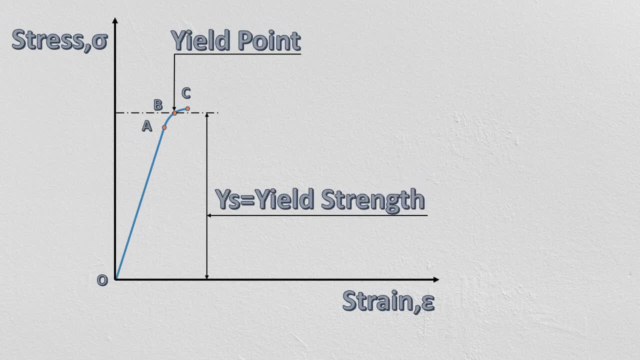 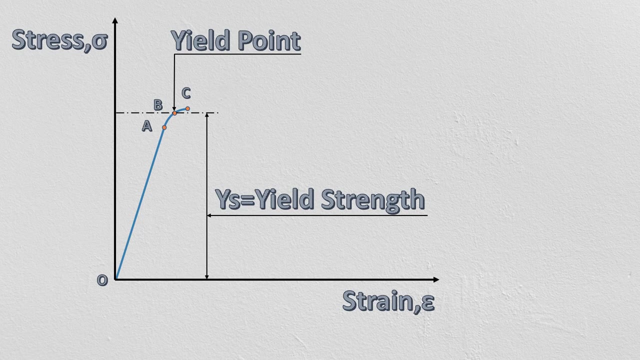 And the corresponding stress value is known as yield strength of the material. When the metal is strained beyond the yield point in the region B- C, the material experiences a change in its crystalline structure and apparently becomes stronger and more difficult to deform. Thus, an increasing stress is required to produce additional plastic deformation.